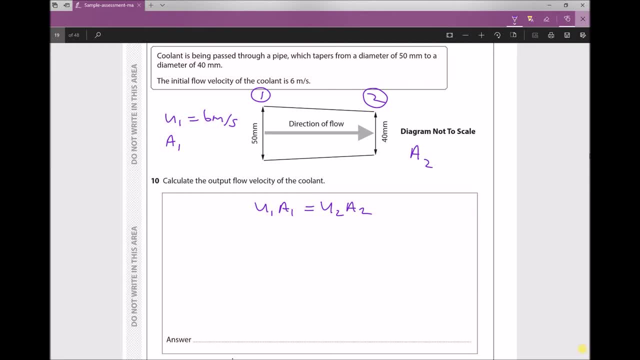 A2.. And in doing so, we'll be able to calculate the outlet velocity, U2.. Let's refer to our equation: U1, A1 equals U2, A2.. We're trying to calculate U2.. So we need to. 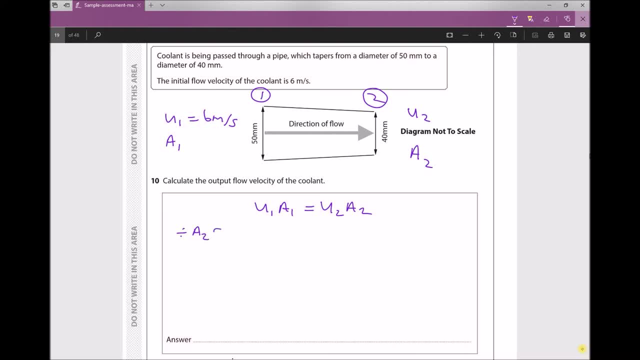 divide each side by A2. And in doing so we will get U2, the thing we're trying to find equals U1, A1 over A2.. Now the area of a circle. we know that this is a circular inlet. 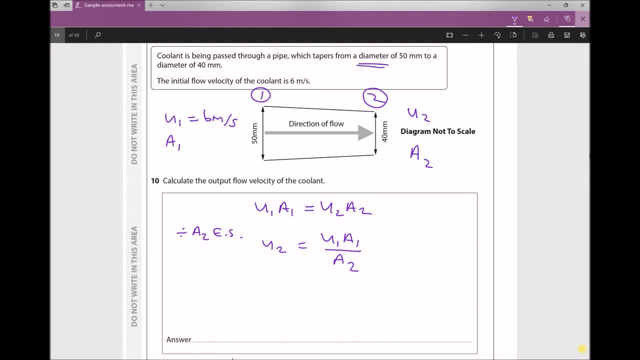 because the question specifies that we have diameters. The area of a circle is pi R squared. So over here, where we've written A1 for the inlet, we know that that's pi times R1 squared because it's the inlet radius, And we know that A2 is pi times R2 squared. 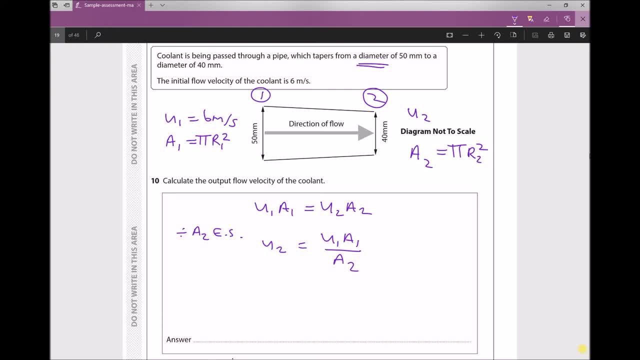 Now, the other thing that I always try to enforce is that we should be working in meters. We need to take our diameter of 50mm and we need to convert it to a radius in meters. So let's write: R1 equals the radius is half the diameter, so 25mm. but in order to 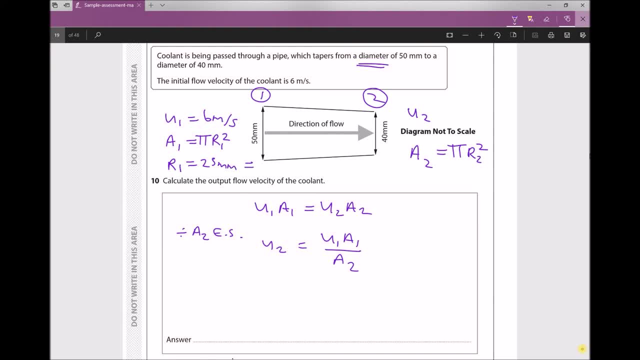 work in meters. I need to divide that by 1000, so 0.025m, And I'm going to do the same for R2.. R2 is going to be pi, R squared, because it's a circular inlet, so square and pi and. 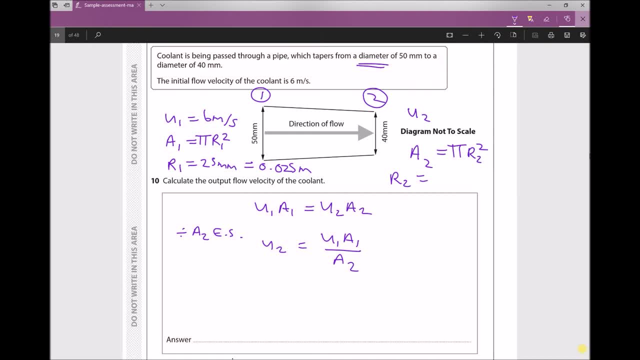 there's going to be pi 0.05m, So en М2 as well multiply and it's just going to add up to some data and then going to be 20 millimeters, because it's half the diameter and 20 millimeters in. 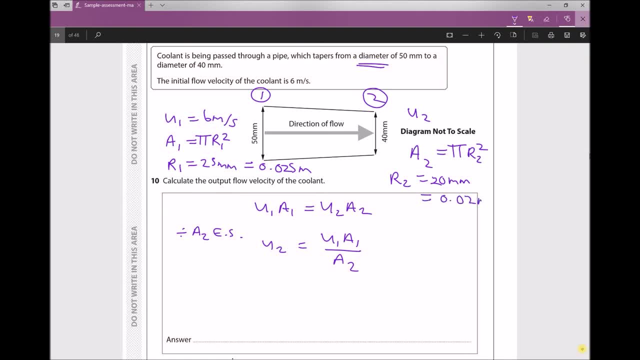 meters is naught point, naught two meters. okay, so now we have all of the information we need, because u2 equals u1 times a1, and we've already said a1 is pi r1 squared divided by a2, and we've already said that a2 is pi r2 squared. so